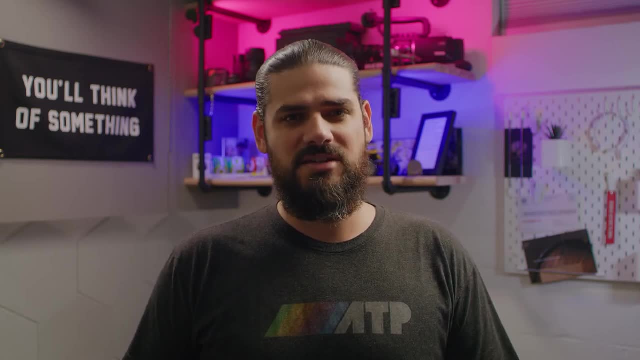 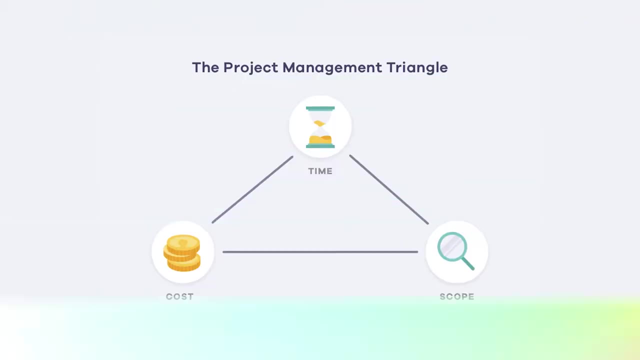 it's your job to balance these triple constraints and manage expectations so everyone understands what it takes to achieve project success. The triple constraint theory is often referred to as the project management triangle. Each side or point of the triangle represents the triple constraints of project management: scope, time and cost. 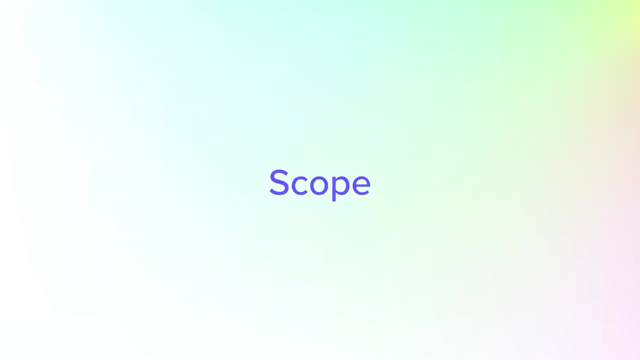 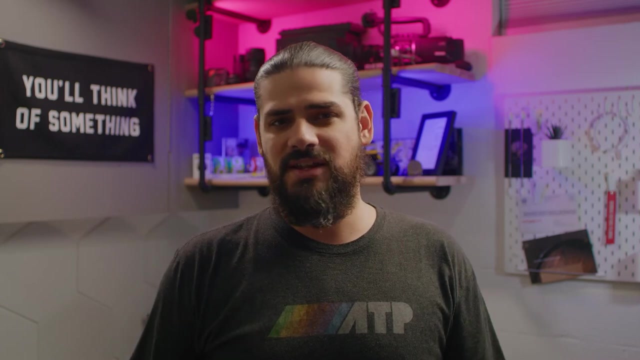 Let's dig a little deeper into each constraint. Scope creep has a funny way of sneaking up on you. Before you know it, just one more thing has turned into a completely different project deliverable. That's why it's important to define and document project goals and requirements before 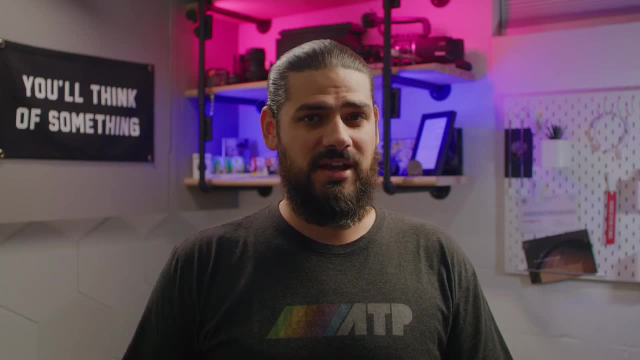 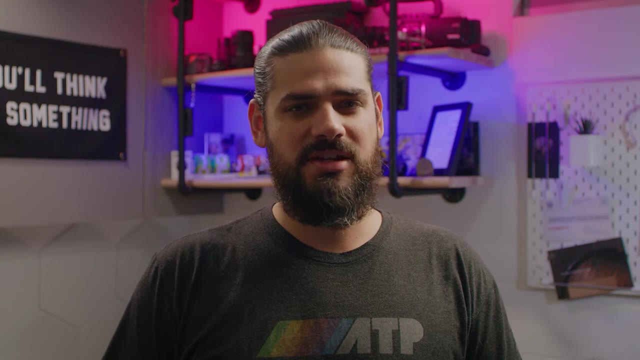 work begins. That way, everyone knows what done looks like and you have a project truth to refer back to. if the scope starts to creep, Adding more features can stretch a project's time and budget constraints. You'll either need to extend the scope to the project or you'll need to extend. 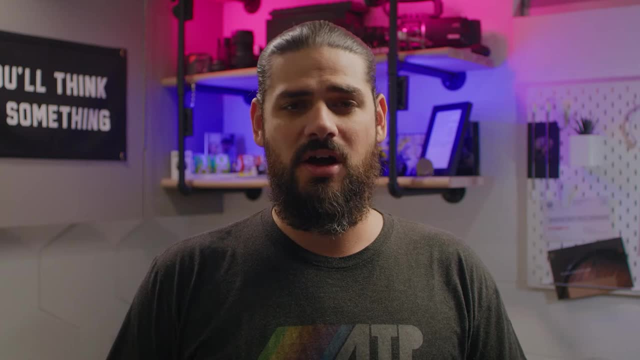 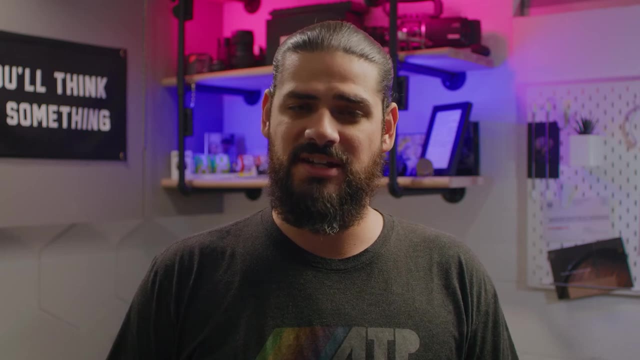 the deadline or assign more people to the work, increasing project costs. Monitoring scope changes enables you to discuss trade-offs early and make necessary adjustments before your project gets off course. In project management, most people know if you want a project done fast, it's going. 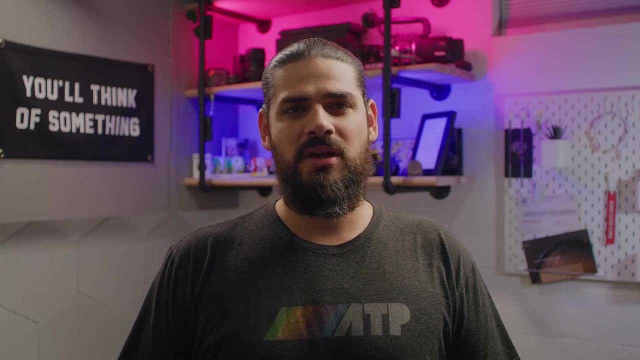 to cost you, especially if you're not willing to bend on the scope. That's because a short deadline requires more resources to get the work done on time. A detailed scope document provides the perfect foundation for understanding your project's goals and wants to achieve a success in the future. 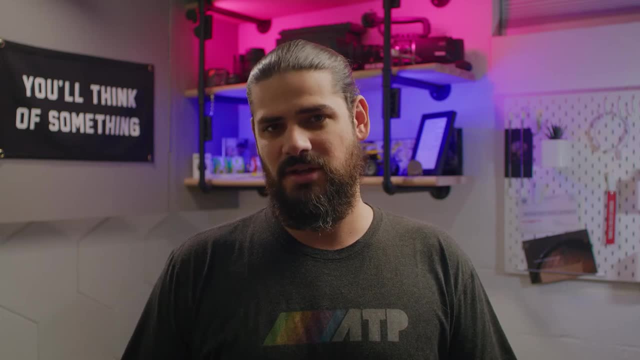 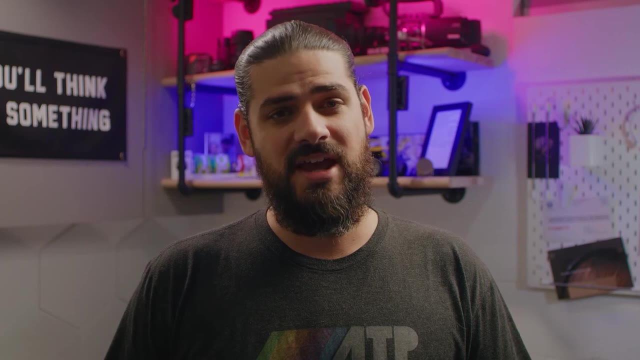 time constraint because you can use it to build out a project estimate. Be sure to bring your team into the discussion and look beyond task hours. The time you spend in meetings or holding a stakeholders hand through the process counts too. The more accurate your estimate, the better. After all, it's what 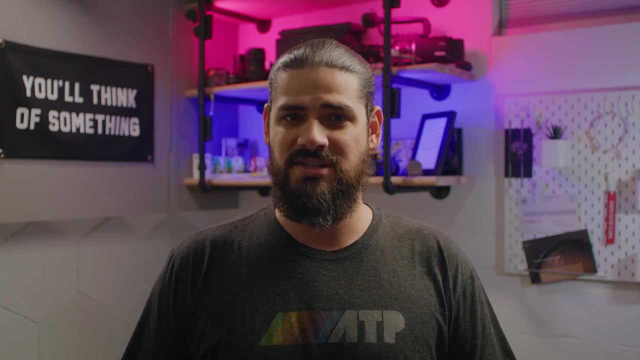 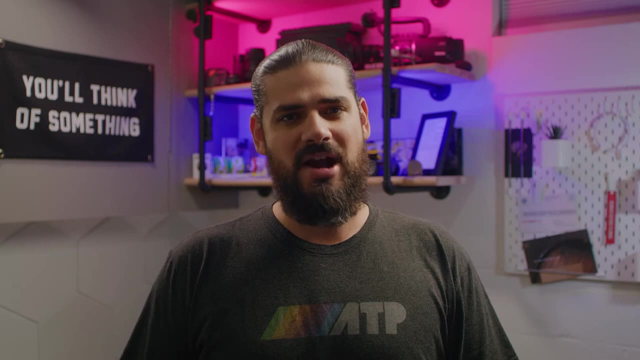 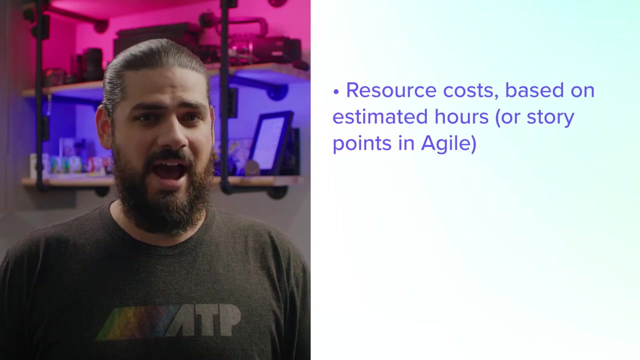 you'll use to schedule work and drive project decisions if tough choices need to be made to meet the project deadline. Estimating a project's time and effort also forms the basis for your project budget. Here are a few costs to consider when formulating a project budget: Resource costs based on estimated hours. 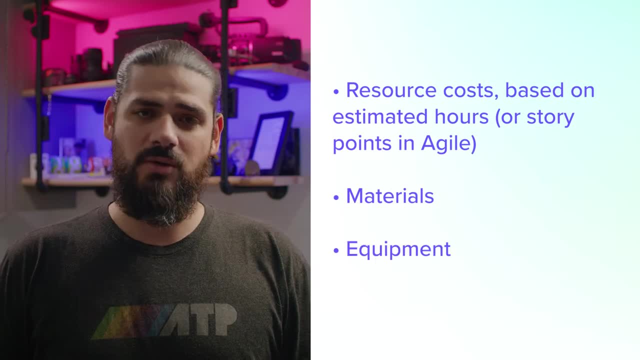 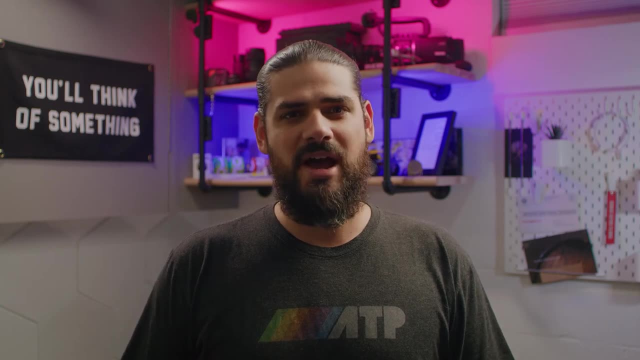 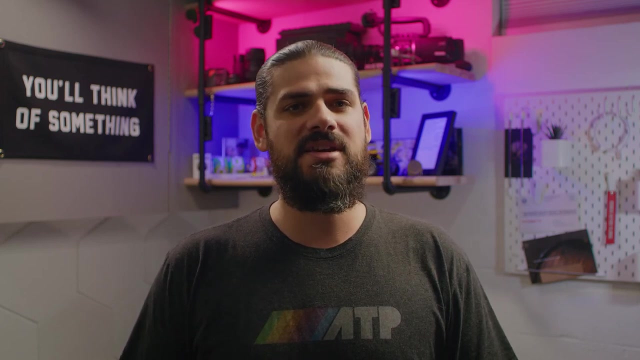 or story points in Agile Materials and equipment. When it comes to budget constraints, remember it's best to communicate early, and often No one likes being surprised by a big bill or the tense conversation that inevitably follows. If an unexpected expense does pop up, take time to explain how it will. 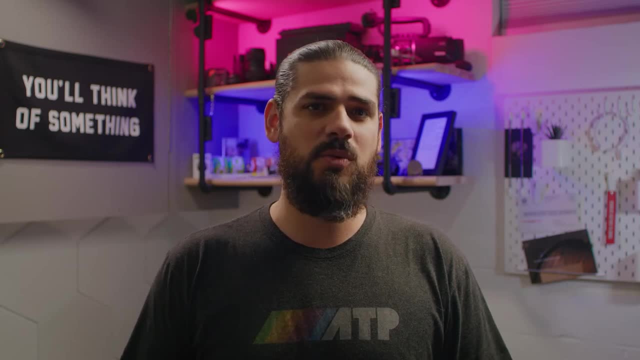 impact the rest of your project and let your client decide whether it's worth it or not. Your client isn't a project expert and may not know what to expect. If your client doesn't know what to expect, they may not realize how much that shiny new feature will cost them in the 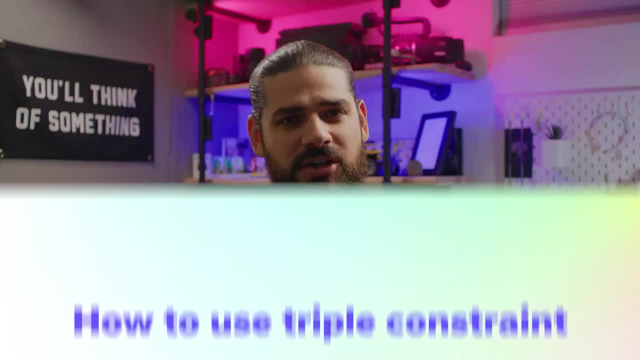 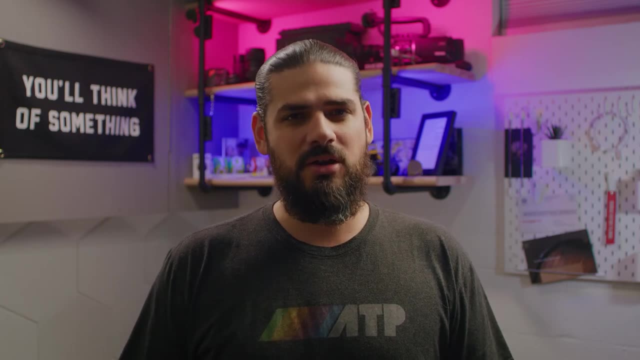 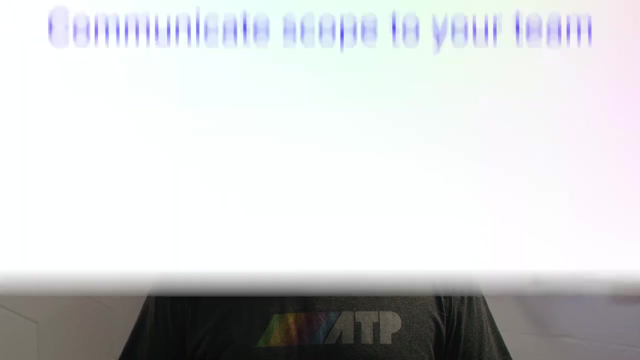 end. Triple constraint theory is all well and good, but how do you put this project management framework into practice? It's all about keeping your eye on the ball. Here are a few ideas on how to use the triple constraint theory to manage a project, using our favorite project management tool as an example. 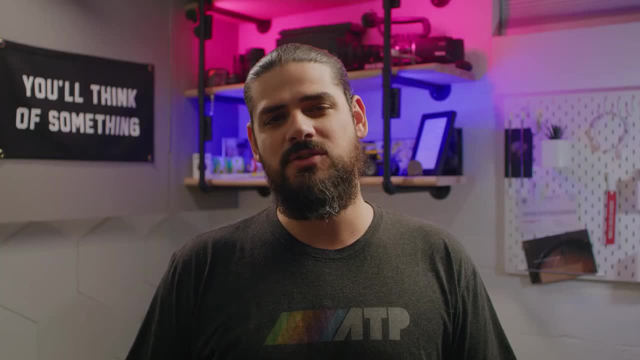 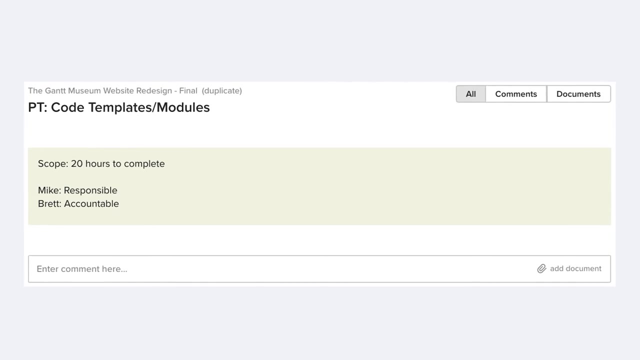 Keeping the nitty-gritty scope details all to yourself doesn't do anyone any favors. Using TeamGantt's sticky note feature to outline scope requirements on the task or project level not only ensures your team has crystal clear direction, it also empowers them to raise a flag if they see the scope start to. 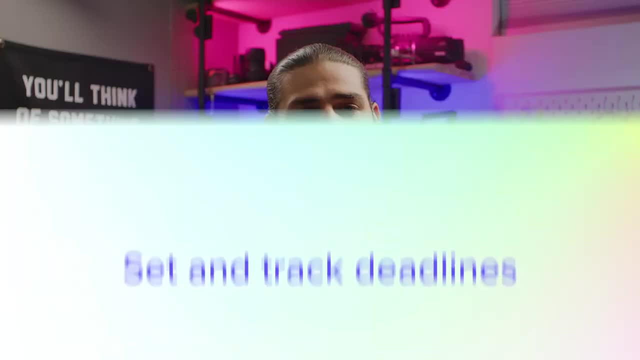 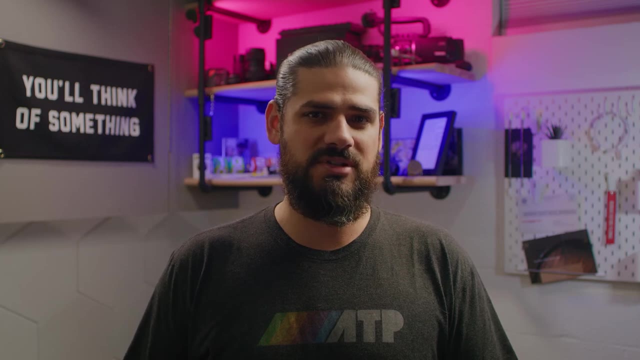 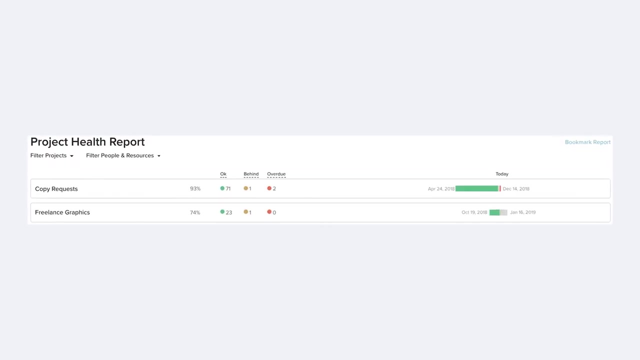 creep. A Gantt chart makes it easy to build and monitor your timeline to make sure your project finishes on schedule. Add milestones to highlight important dates and deliverables, and use baselines to compare your planned versus actual timeline as your project progresses And if you want a quick snapshot of project. 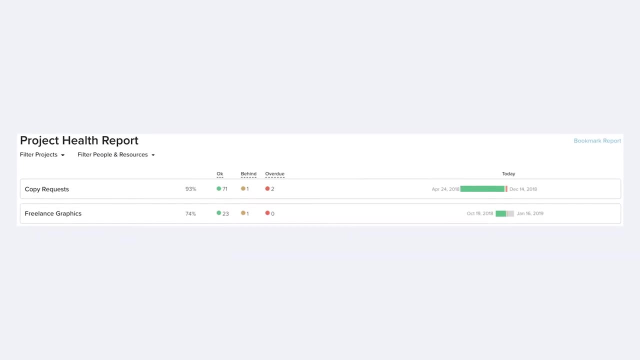 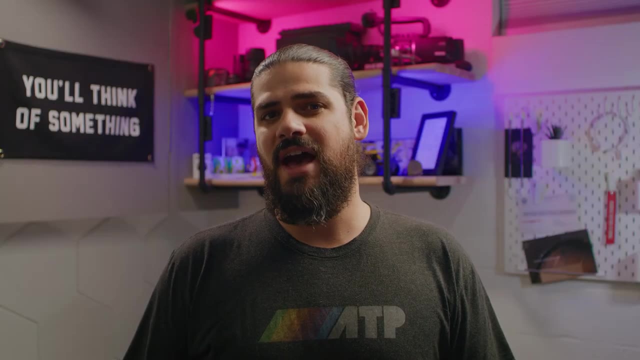 delays. TeamGantt's project health report shows you which tasks are falling behind and which ones are already overdue. Time is money in any project-paying attention to how the time spent stacks up against your estimate helps you keep project costs in check. TeamGantt's hourly estimation and time tracking. 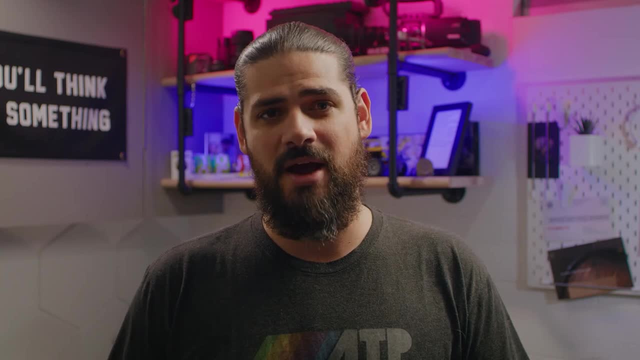 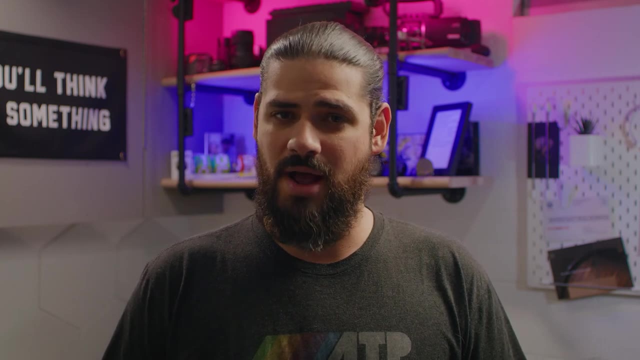 tools enable you to compare a tasks- actual vs estimated hours and see how the time spent tracks against the percentage complete. That way you can spot budget overages before they become a problem. If you want to win at project management, you've got to be a pro at wrangling scope. 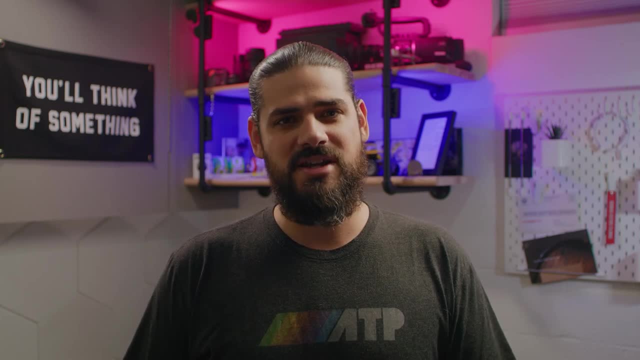 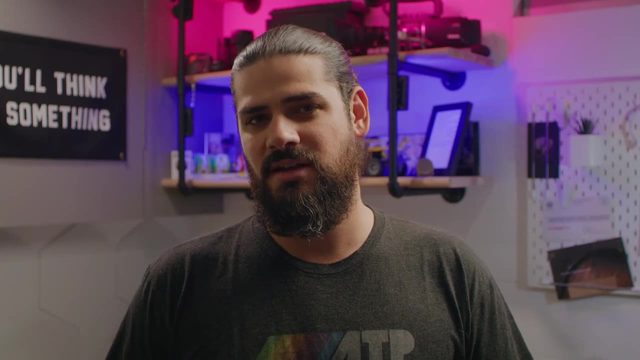 time and cost. With TeamGantt, it's easy to balance project constraints, so everyone's happy with the outcome. You'll have all the features you need to ensure projects finish on time and under budget. Best of all, it's all wrapped up in a 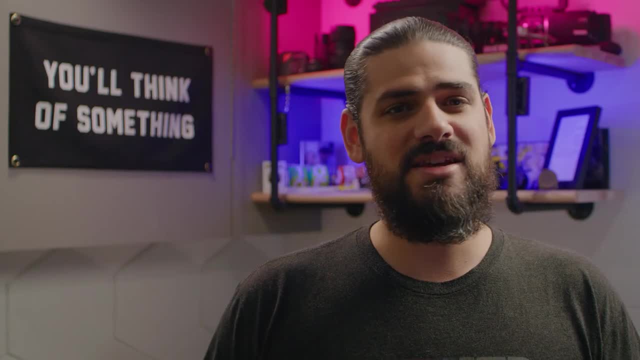 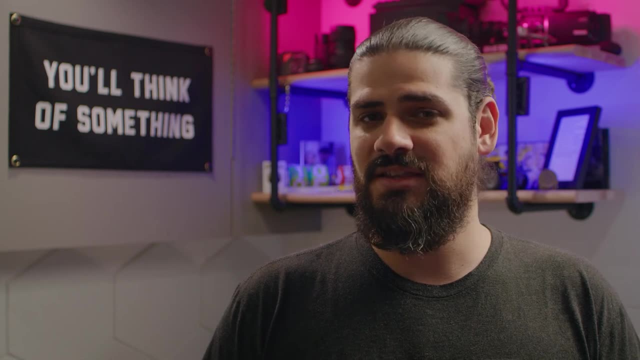 simple, intuitive interface. anyone can navigate. And that's it for this video on triple constraint project management. I hope you found it helpful. If you did, I'd love it if you could return the favor and hit the like button. And don't forget. 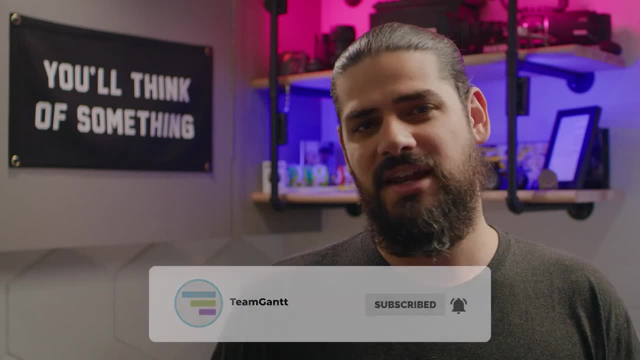 to subscribe to our channel and turn on notifications so you don't miss any of our videos. Thanks for watching. I'll see you next time.